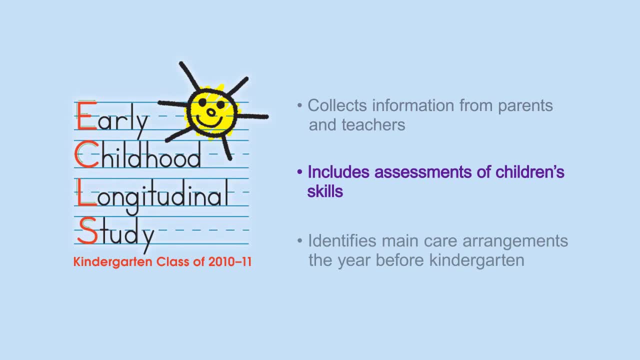 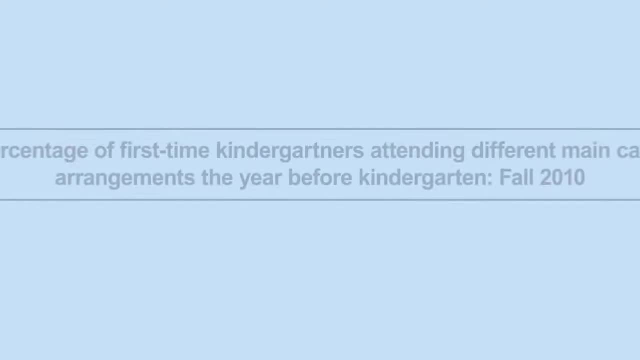 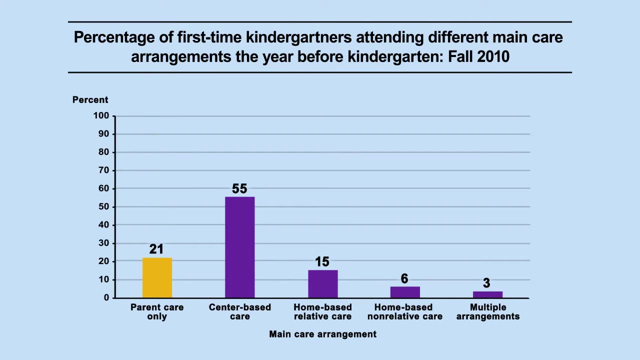 fifth grade and includes assessments of children's skills. Parents reported on their child's care arrangements the year before kindergarten. One percent of children who were first-time kindergartners in the fall of 2010 received care only from their parents on a regular basis the year before kindergarten. In comparison, 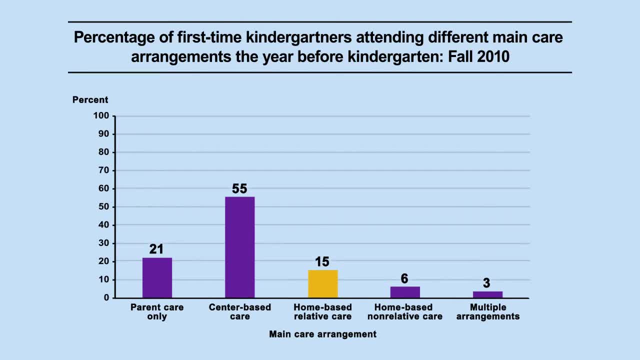 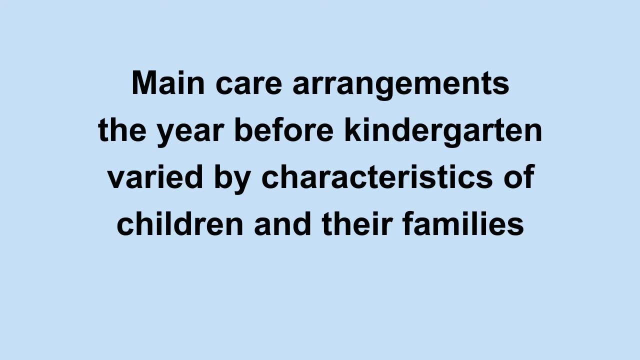 fifty-five percent were mainly in center-based care, fifteen percent were in home-based relative care, six percent were in home-based non-relative care and three percent were in multiple arrangements for equal amounts of time. Main care arrangements the year before kindergarten varied by characteristics. 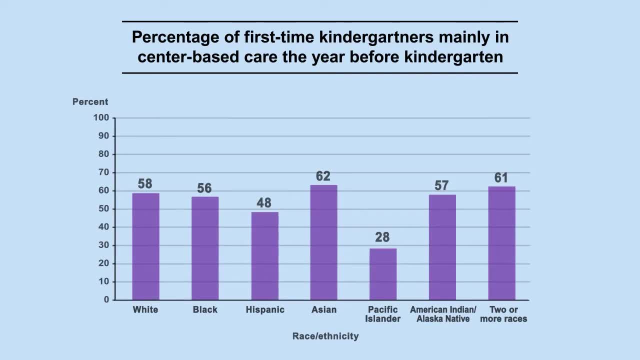 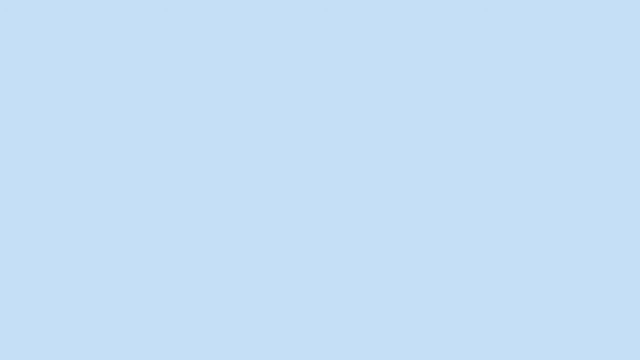 of children and their families. For example, the percentages of Hispanic and Pacific Islander children who were mainly in center-based care were lower than the percentages of children from other racial ethnic groups. Another characteristic of interest is children's household socioeconomic status, or SES, which 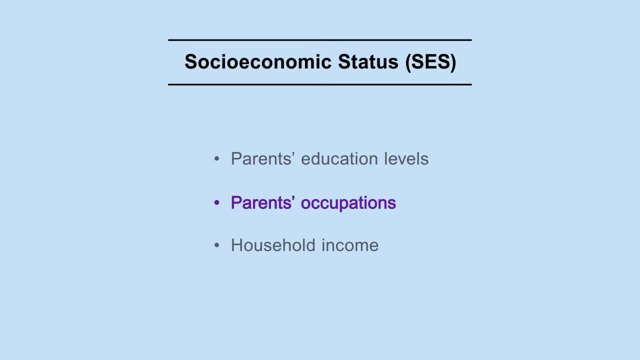 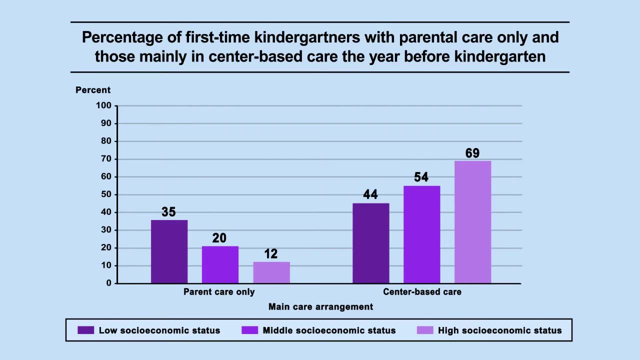 was based on their parents' education levels, occupations and the household income. It was more common for from low SES households than for those from higher SES households to receive care only from their parents the year before kindergarten. In contrast, it was more common for children from high SES households than those from lower SES. 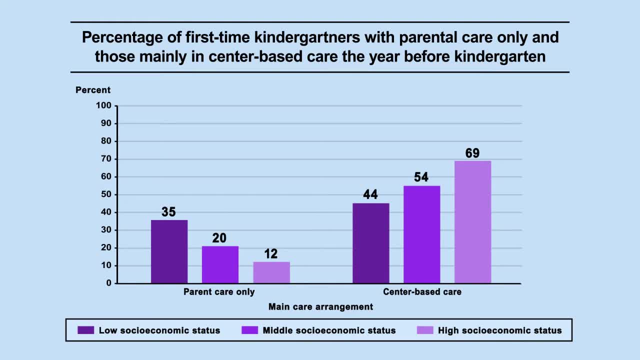 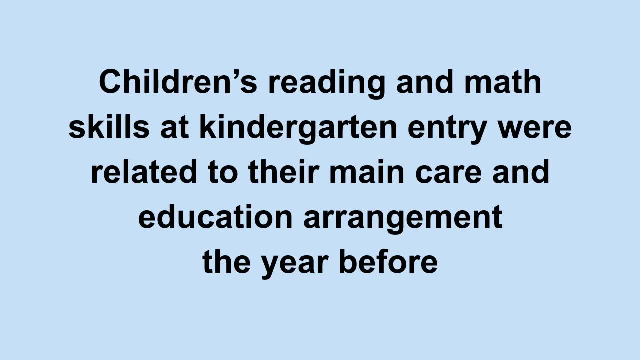 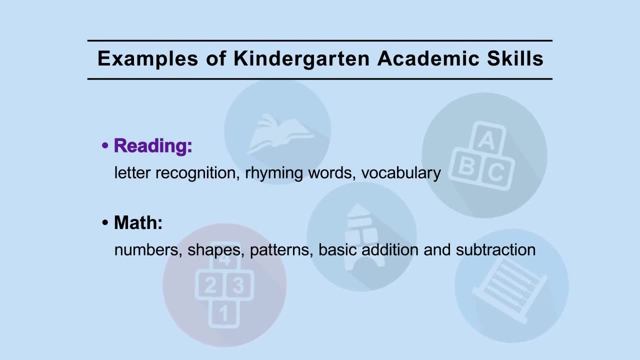 households to attend center-based care as their main arrangement. It is also possible to explore whether children's reading and math skills at kindergarten entry were related to their main care and education arrangement. the year before The kindergarten reading assessment measured basic skills like letter recognition, rhyming words and vocabulary. The math assessment measured 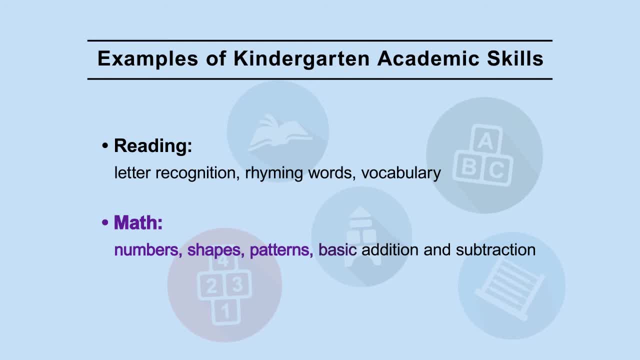 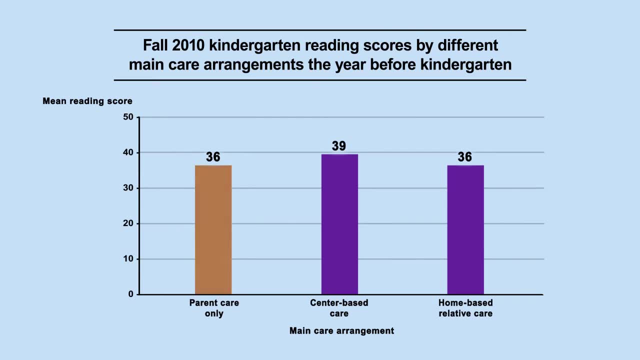 concepts like numbers, shapes, patterns and basic addition and subtraction. In 2010,, children who had only received care from their parents the year before kindergarten and those who had been mainly in home-based relative care scored lower in reading at kindergarten entry than their peers who had